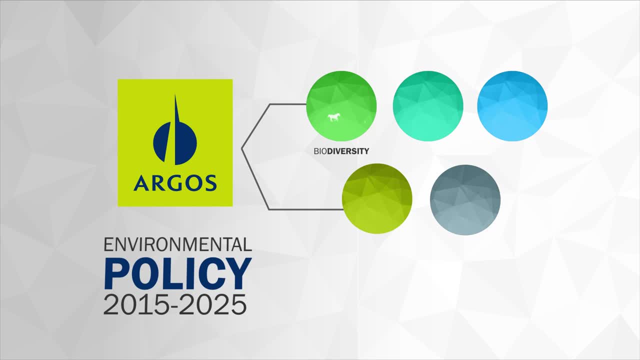 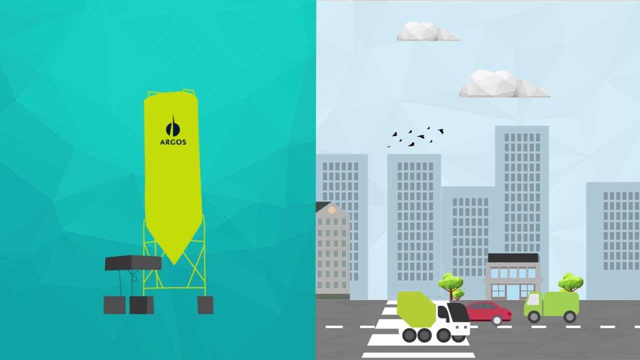 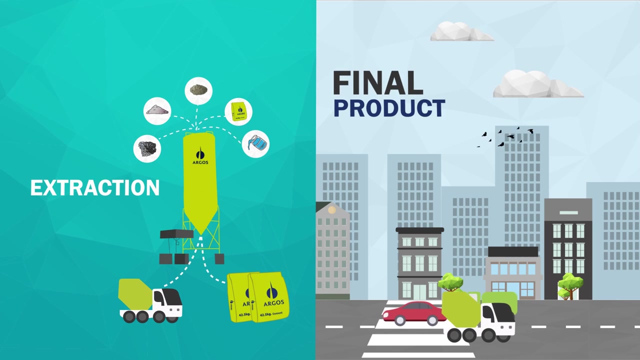 towards 2025, focused on five pillars: Biodiversity, climate change, eco-efficiency, sustainable construction and the environmental element in Argos' culture. These pillars are the outcome of a study of our main environmental impacts that cut across the entire operation, from sourcing raw materials to the delivery of our products, Taking into 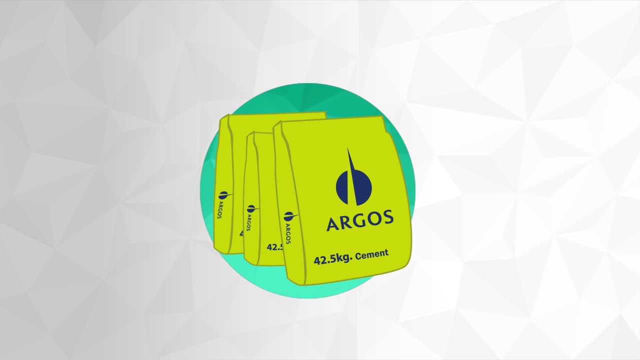